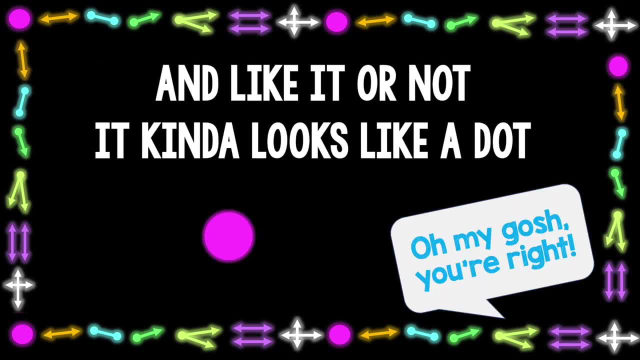 In space, in liquid or not. it kind of looks like a dot. Oh my gosh, you're right. Join it to the end of a line and guess what it's called. I don't know. an end point, That's right. 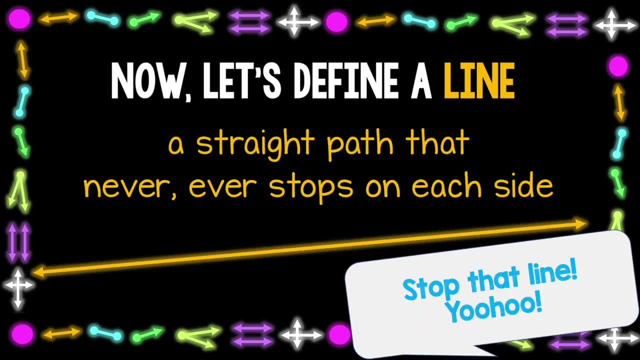 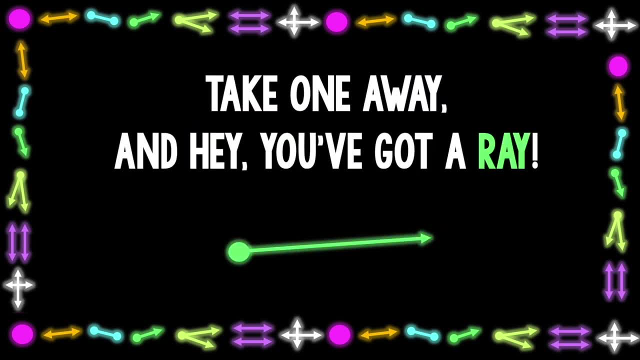 Now let's do it. A straight path that never, ever stops on each side. Stop that line. yoo-hoo, A line segment will help your dreams come true. Smack attack with two end points on the back. Take one away and hey, you've got a ray. Bring all two rays or line segments together to form an angle. There's. 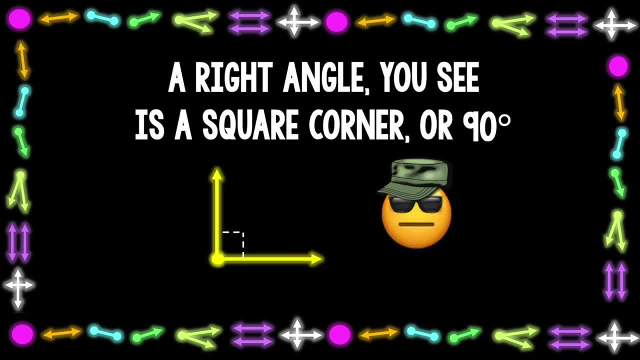 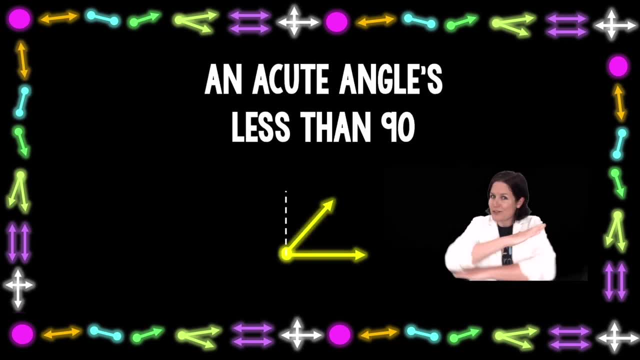 some angles that you need to know: Right, acute, obtuse and straight are the four. The right angle, you see, is a square corner or 90 degrees, And acute is so cute, like a little baby, And acute angle is less than 90.. Yo, dude, I'm obtuse. Uh, how did he get up to this? I don't know, I don't. 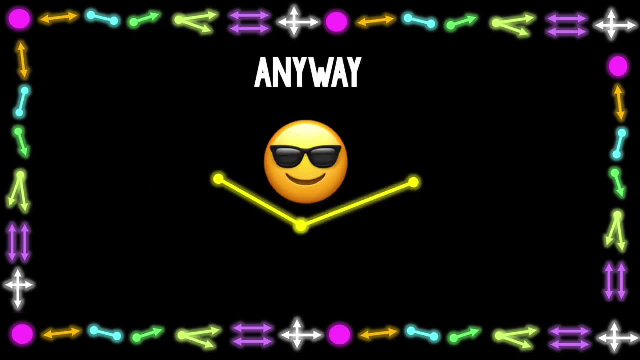 get loose. Excuse me, some people think I'm cute too, Geez. Anyway, I'm wider than a right, with my arms open, wide, ready for the best hug you've ever had in your life, Right? Oh, it's not up for debate. 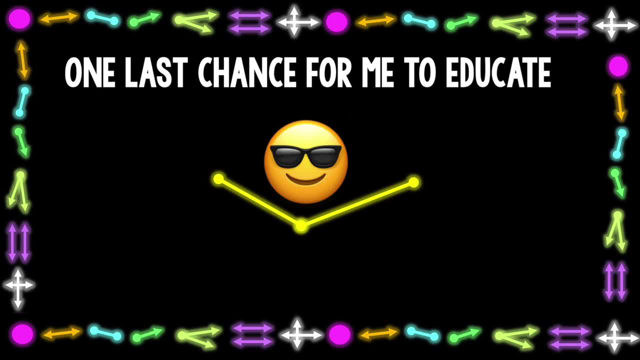 My hugs are great and hey, I'm late for a date. Oh wait, one last chance for me to educate. He's kind of overrated. Everybody needs straight. Wait. a straight line is an angle 180.. Don't get your. 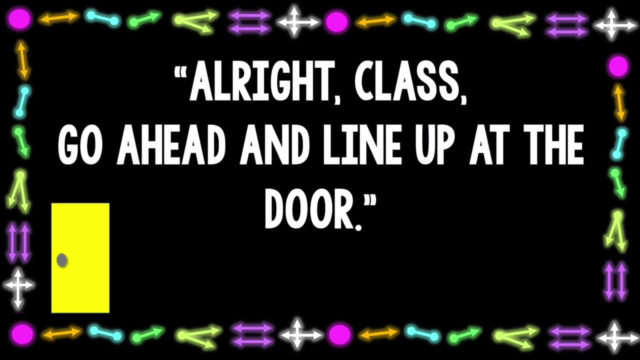 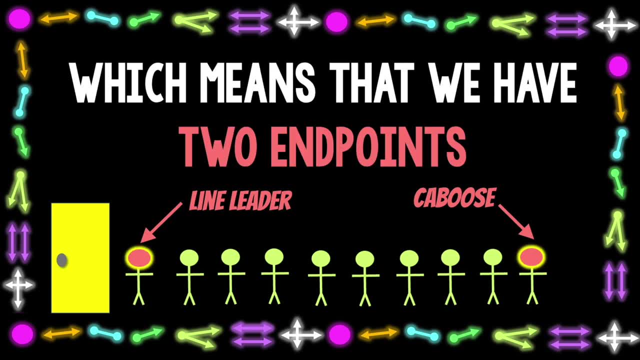 angles tangled. So I was thinking: you know how teachers they say: all right, class, go ahead and line up at the door. Well, hold up a sec, because we've got a line leader and a caboose at the end, which means that we have two end points. That's not a line. So maybe next time the teacher should. 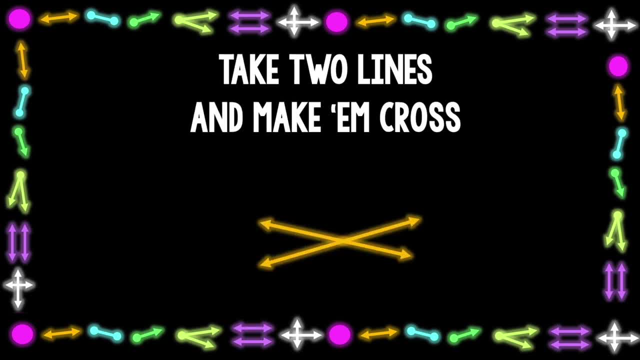 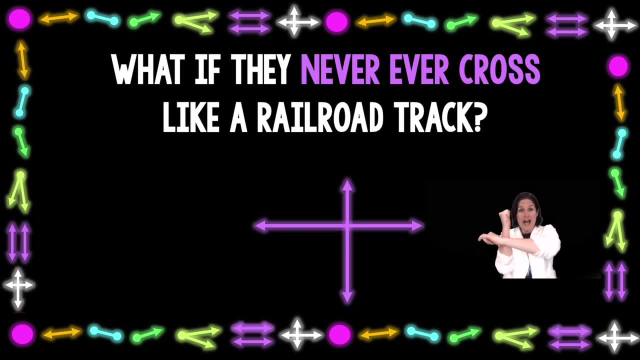 say, line segment up, Take two lines and make them cross. Now they're intersecting, Crisscross. If they intersect and make angles, that are right Perpendicular lines, But if they never ever cross like a railroad track, That'd be swell, if there was well a special name for that. Well, consider, 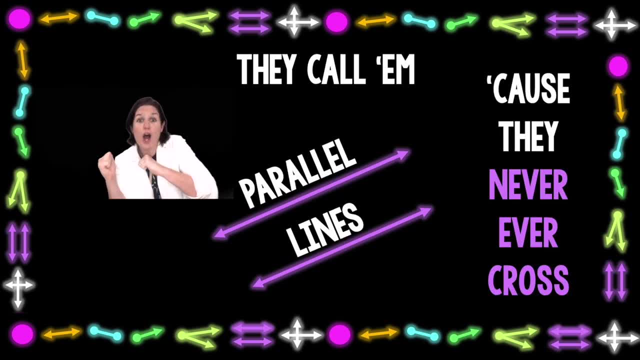 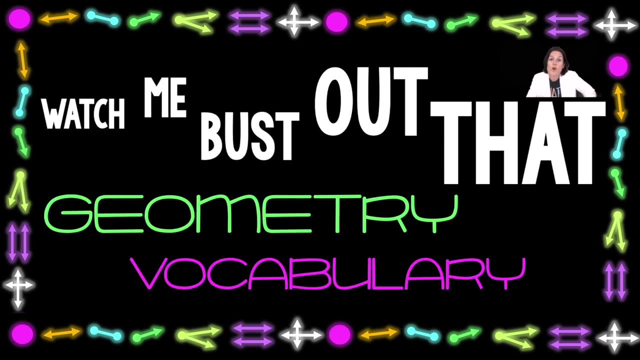 this your lucky day, boss. They call them parallel lines because they never, ever cross. You know, I love me. know, I love me some geometry. Watch me bust out that geometry Vocabulary. You know, I love me. know, I love me some geometry. Watch me bust out that geometry. 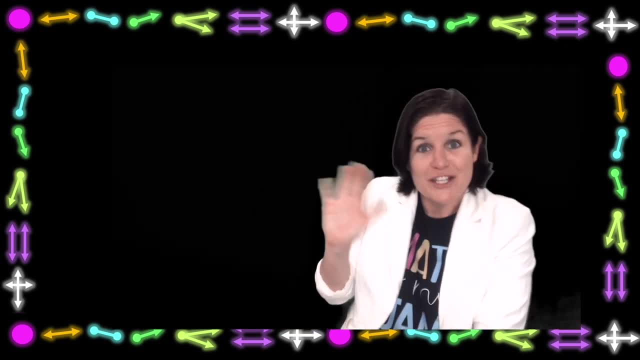 Vocabulary: See you in part two.